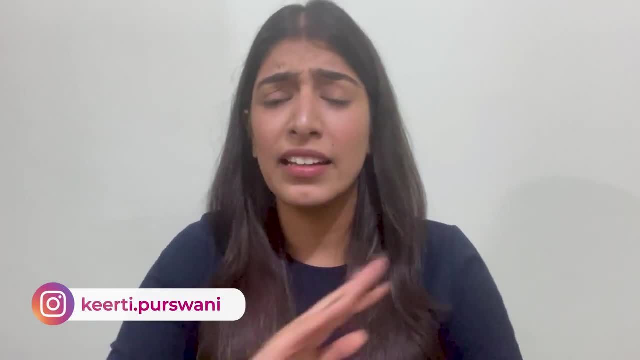 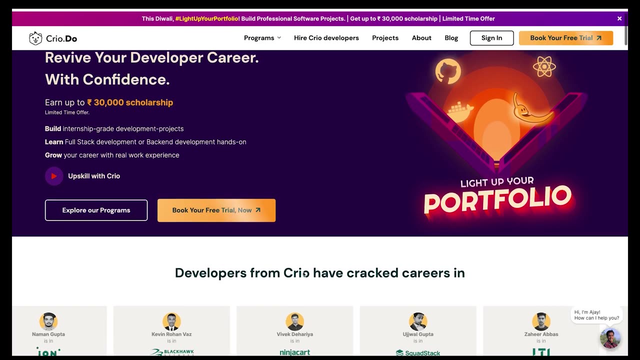 to see why do we need factory design pattern, how to implement it and everything in detail. But before we get started, let me tell you about the sponsor of the video. Cryo is a project-based learning platform. They have a fellowship program that comes with either of the two programs. 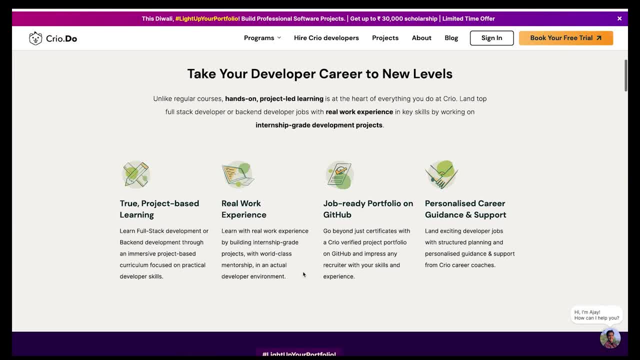 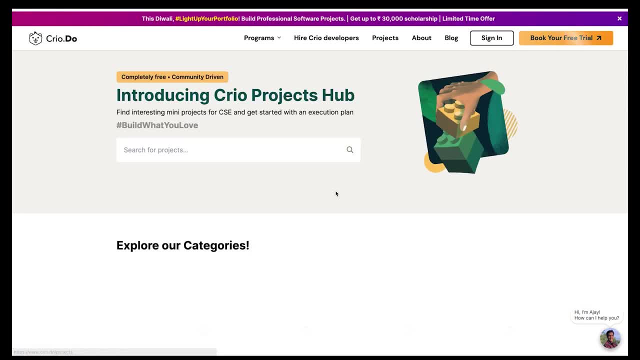 that is, the full stack or the back-end development, and it guarantees you a job. along with it, You can get a job from 6 LPA to 18 LPA. They prepare you for all kinds of interview questions that you can come across, and they also are offering a scholarship of 30,000 on this. 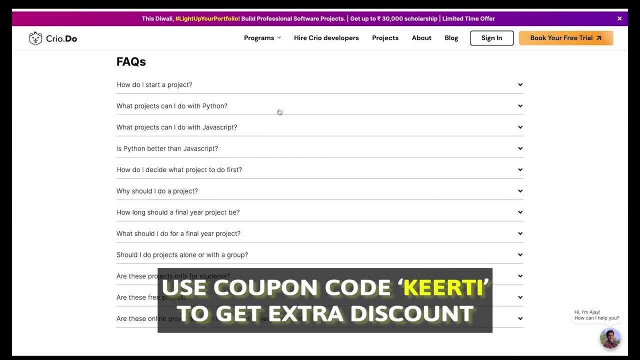 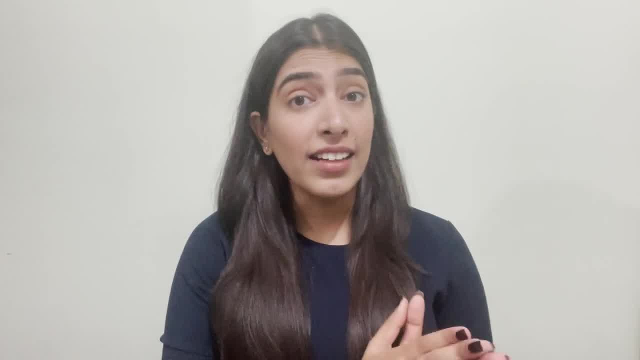 program. So do check it out and don't forget to use the coupon code Kirti for additional discounts. You might really like those. Let's start with a very basic example. So there's a client. the client has asked you to create a vehicle library Basically. 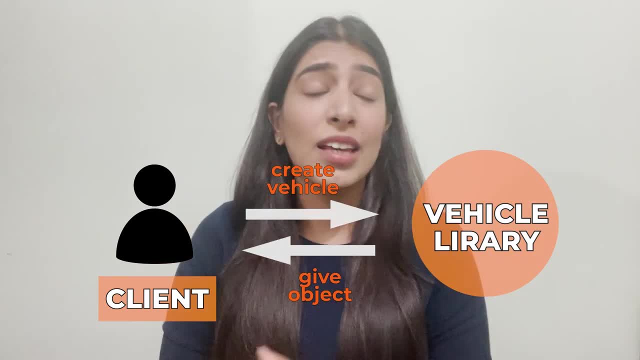 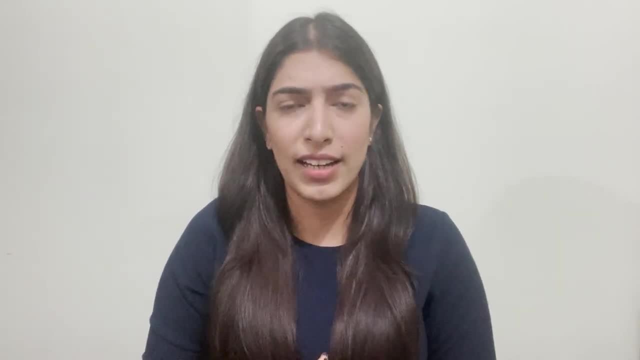 you're supposed to create vehicles and give back to the client. Now, a vehicle can be a car, it can be a bike, it can be a bus. Client is just going to tell you: I want this particular vehicle. you create it and you give it back to the client. Very simple thing. This is a very basic day-to-day. 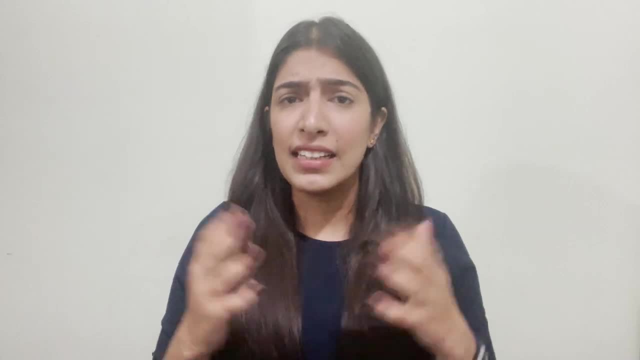 example right. So now, since you know oops, you're going to say Kirti. this is very simple. This is basics of oops. We are going to create a base class vehicle and we are going to inherit. 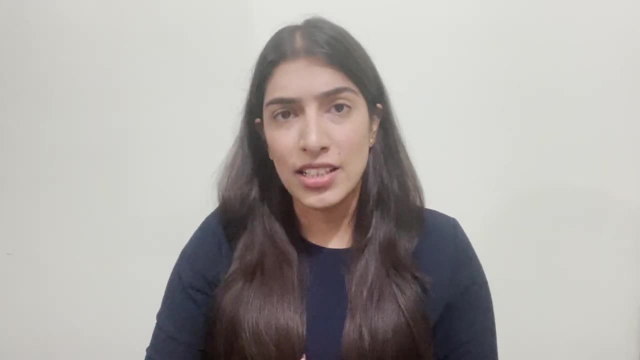 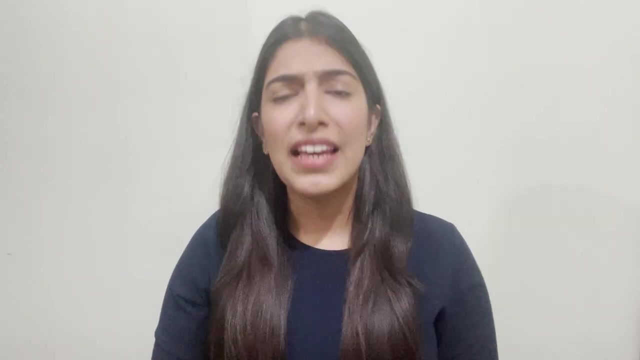 class's car class's bike bus, whatever is there from the class vehicle. right, Let's do this much thing for our client and let's see what will be the wrong thing with it. Let's just start writing the code. So I'm going to start writing the first class, our base class, that is, the class vehicle. 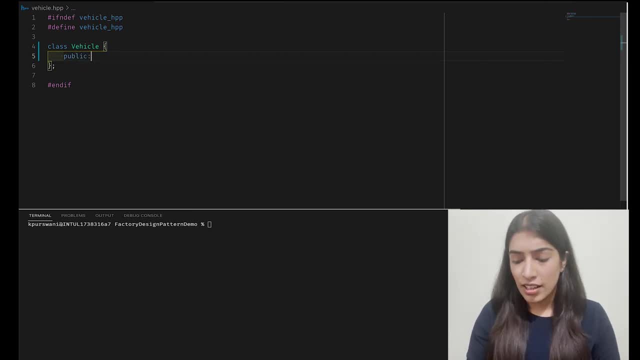 Okay, And I'm going to write for now just one function. I have made it public and I am writing a function. Now, guys, don't get overwhelmed by these virtual void equal to zero and all. I'm going to explain everything in detail, Although I'm 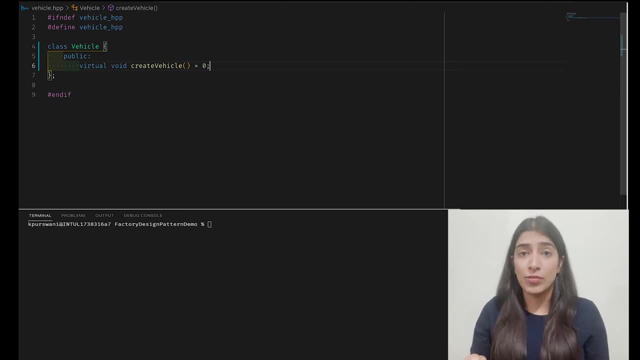 writing the code in C++. the entire concept is completely language independent. I'm going to explain you everything in detail. For example, here I've written virtual, void and equal to zero. Basically, what I've done in C++ is: I've created this particular function. 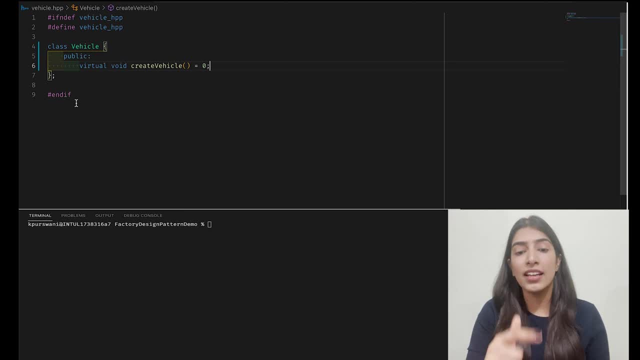 as pure virtual function. That means any class that inherits from vehicle will have to implement this particular function, that is createVehicle. Now I have made this an interface. Now classes that will derive from vehicle, like class class car, class, bus, 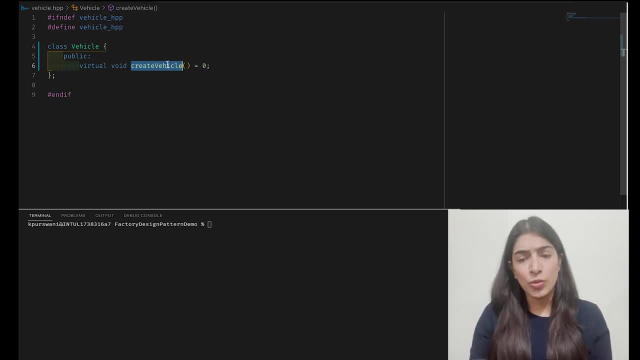 will have to implement this function for sure. that is what we wanted. that is what I have done, very simple, okay. so now we have written the class vehicle, we are going to write two more classes: class car and class bike. we are going to inherit from this class vehicle. okay, so here I am going. 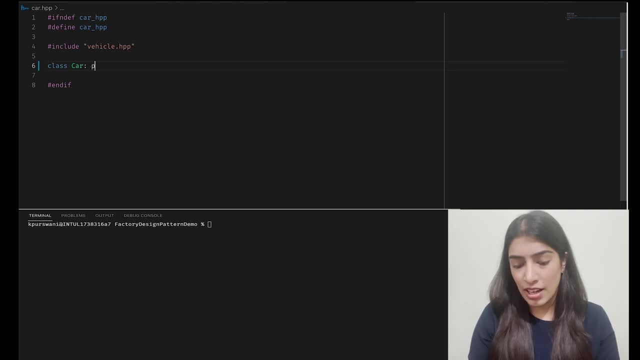 to start writing class car. I am going to inherit it from vehicle and which function will? am I going to write in this the same function that I had written in vehicle? right as you can see, I am writing it in uh HPP files. these are the header files and I have already given the header cards. 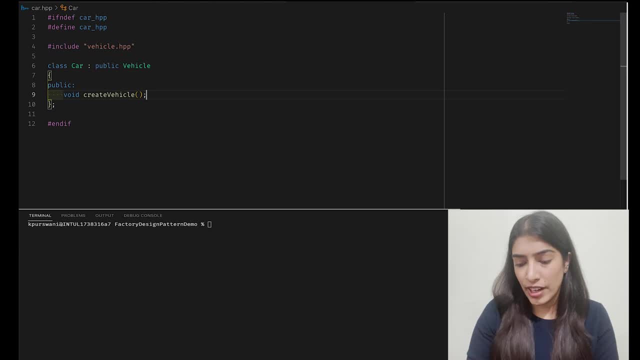 and all. so don't worry about all of that. right so I have defined create vehicle. now the same thing I need to write in the CPP file. right so, right now, in CPP, all I am going to do is like I am going to write an output statements. that's it, alright. for now we are not going into detail, nothing like that. 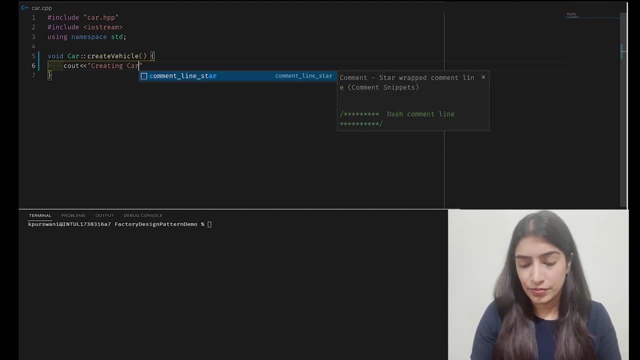 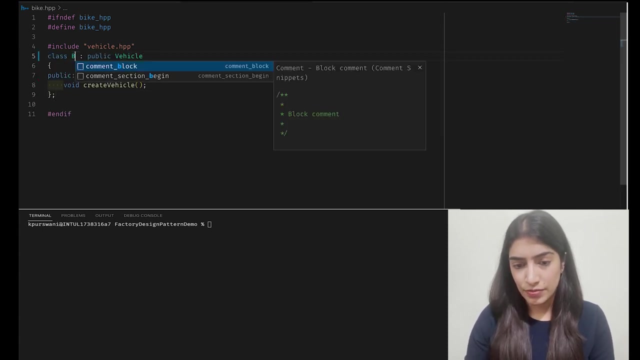 I am just is writing: creating car. now, just like car class, we are going to make one more class class: bytes. this is just for example purposes. okay, same thing. so from carhpp, i am going to copy the code, put it in bytehpp and i'm going to rename this to byte, and that's it i'm going to take. 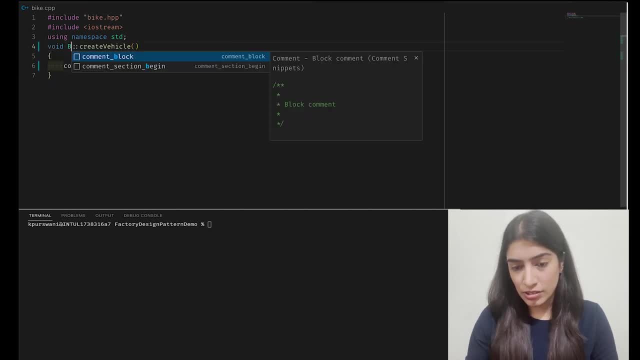 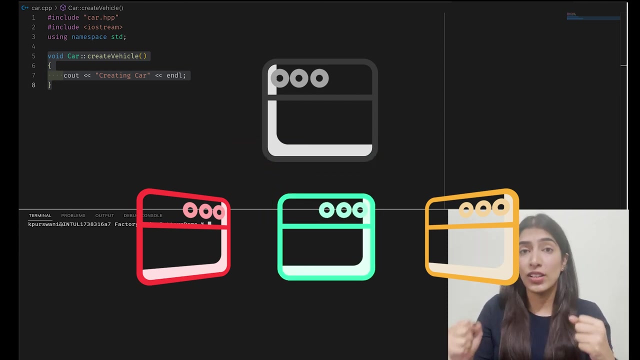 carcpp and put it in bytecpp and i'm going to just write: creating bike. that's it. so what have we done till now? we have created a class vehicle, we have created class car and we have created class bike. we have inherited these two classes from class vehicle. right now, let's compile these. 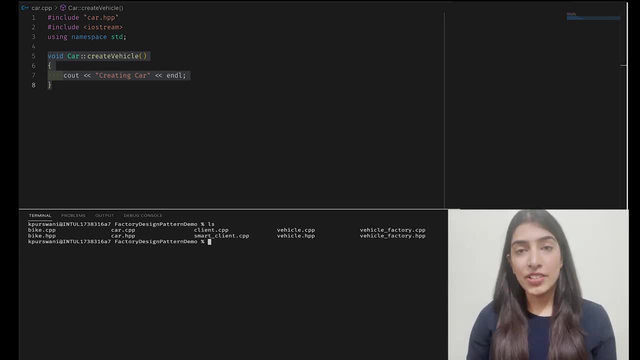 create a library. give it to us simple right. let me first show you what all is there in the folder. okay, right now we have bytecpp, bytehpp, carcpp, carhpp, vehiclecpp, vehiclehpp. let's take care of only these six files, ignore the rest. okay, so right now. 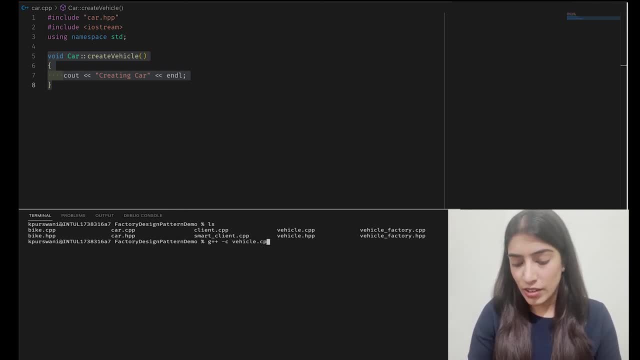 i'm going to compile them and create object files. okay, so i take vehiclecpp, carcpp, bikecpp, and now you can see object files are created for them: bikeo, caro and vehicle. okay, so we have created object files. now we are going to put them in an archive, put them in a library to give it to. 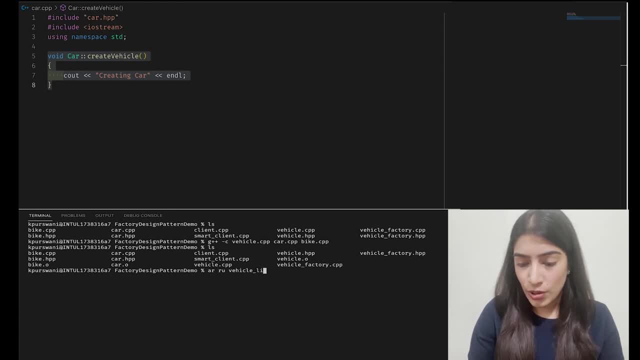 our client: okay, here are you. we are going to call our library as vehicle library, dot a for archive, and then we are going to use the object files, right. so now you can see the library is great. okay, now we can give this to our client. let's write the. 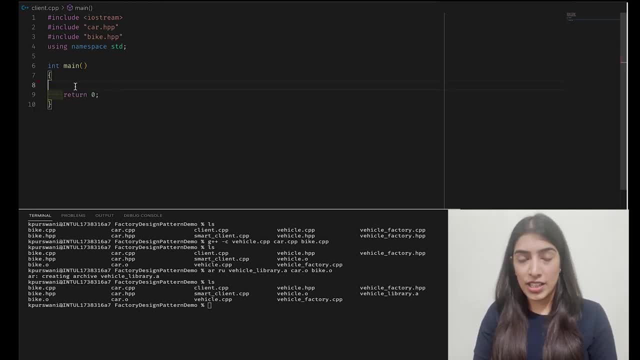 client code now. okay, so this is our client, this main function in this line. what am i going to do? i am just going to type the object you want to call themcpp, carcpp, routinecpp, vehiclecpp, datacpp. and based on this, so if the vehicle type is, say, car, i am going to create vehicle, right, so 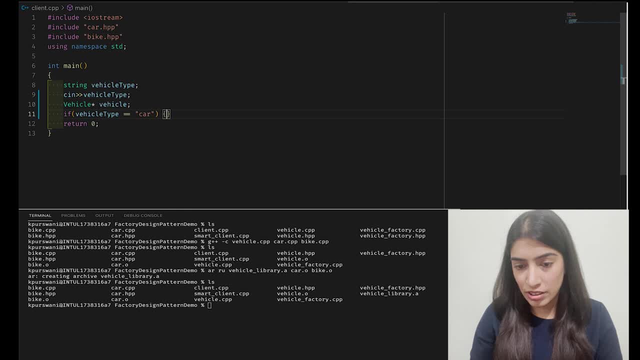 i am going to create vehicle pointer right now, and if the type that i am going to write is carcpp, i want is car, i am going to make this as new car. if i take the input as bike, then i am going to create the bike as it. so i have created the vehicle object. now what am i going to do? i am 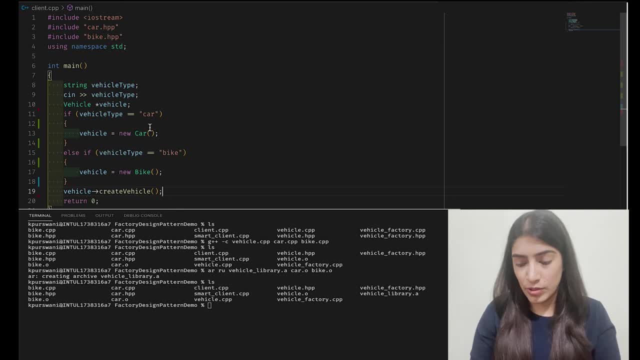 going to call the function create right. so this is our client. just to revise what have i done till now. i took a vehicle type input and i saw that if it was car, i created a class car. if it was by, i created a class by, and i just call this function create right. so now i am going to compile a client. 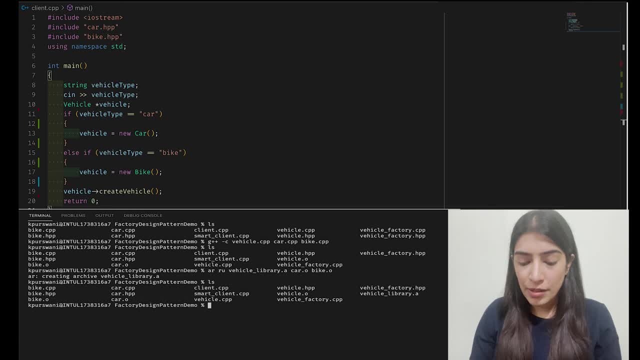 and use this vehicle library to now create the vehicle. i am going to do g plus plus minus o. this is to link and i am going to call our executable as client and i am writing our client dot, cpp and using vehicle library car. okay, so now i can execute my 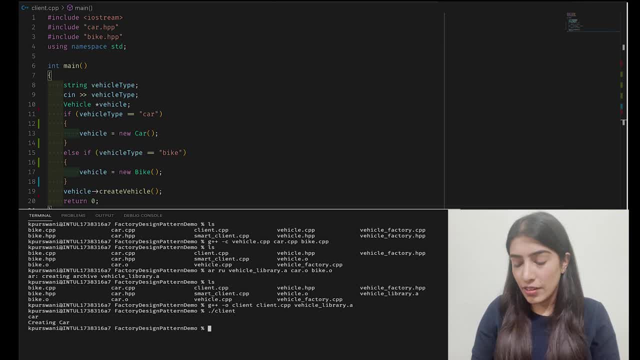 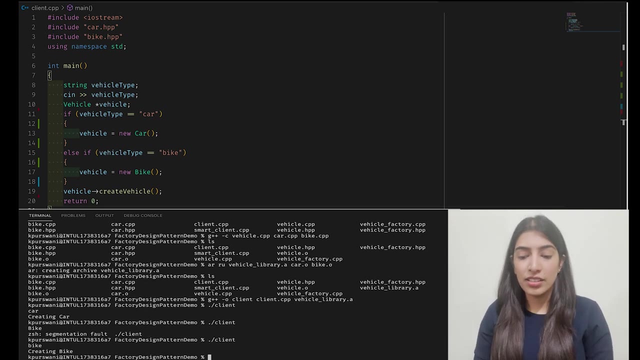 executable client. so if i give the input car, i have, i got the output as creating car right. similarly, if i do y, i have. sorry, i have not handled the wrong input and all. so for now, if i give the bike, i am creating bike right. so now, as you can see, everything will. 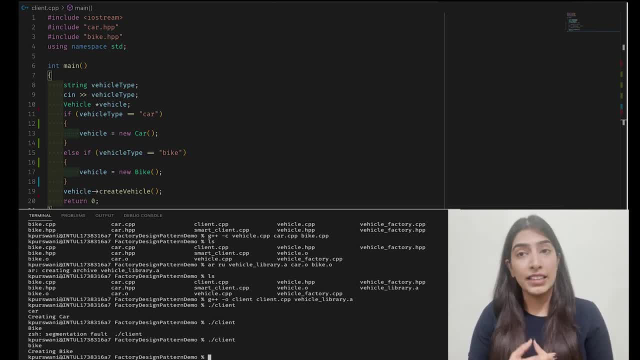 works fine, right, we compile client. if we give the input car, it created car. if we give the input as bike, it created bike. so it works fine. but now let's see what the problem over here is right now, what we did. our library had just car and bike, right. so whenever a client needed car or bike, it 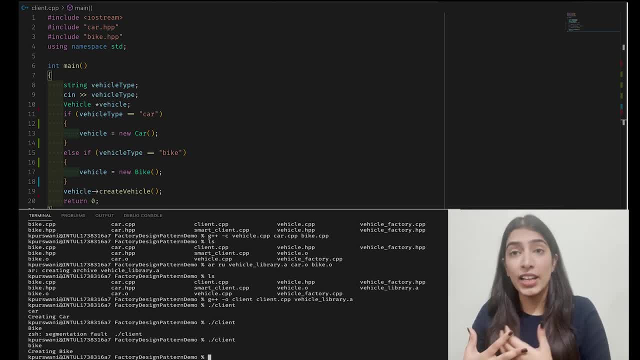 created that right now. tomorrow, if our library wants to extend itself and say that now i am going to give the functionality of creating a tempo or a bus also, not just car and bike, so we add these particular files to our library, what are we going to do? we are going to tell the client. 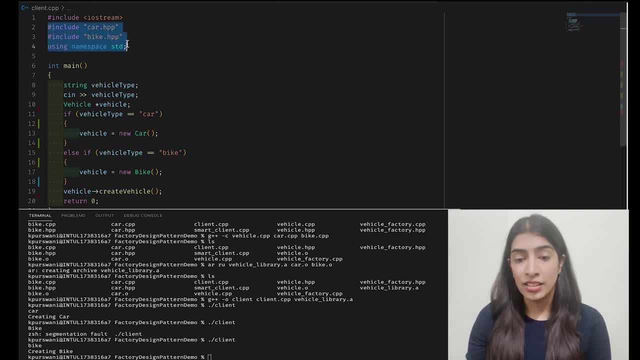 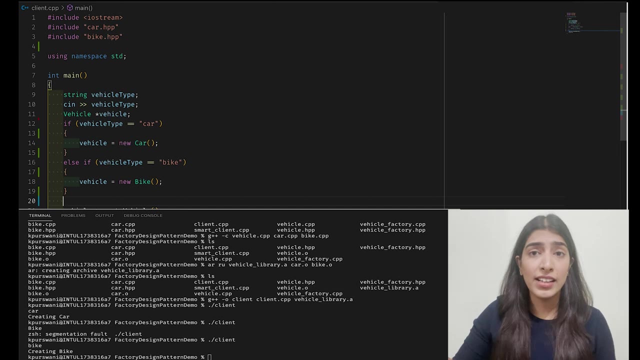 that you know what. right now, you are including only car and bike. right then, after that, if i have already given you bus and truck or tempo, you include these and you add these to your if else conditions. is this right? every time we make any changes to library, we add anything, we are telling. 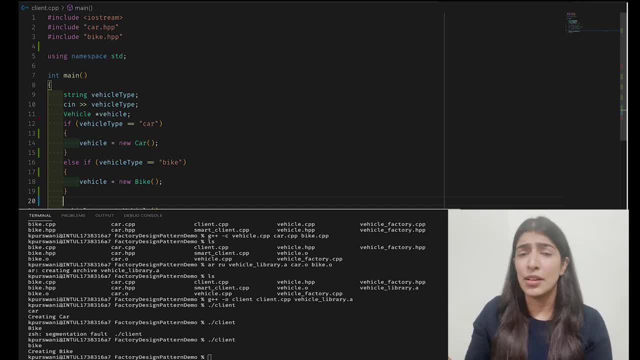 our client. so tomorrow, if we make any changes, we add truck tempo bus, anything thing. we are going to tell our client that you include the hpp files and you add these statements in your if else condition. that is wrong. our client might not want to do it. we are telling 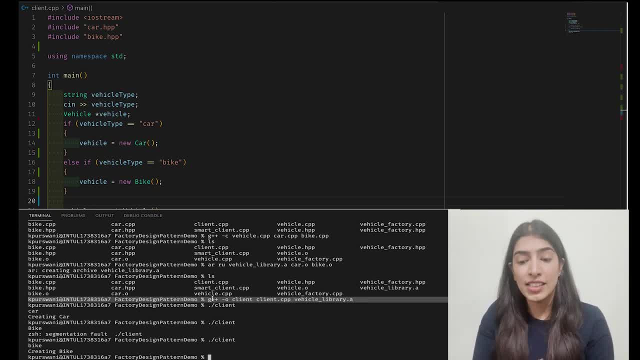 our client. you will have to compile yourself again and again the last statement that i did that you know we use the clientcpp to create the executable client right, but when we change the vehicle library it is not always necessary that client wants to change itself at that time. this is very 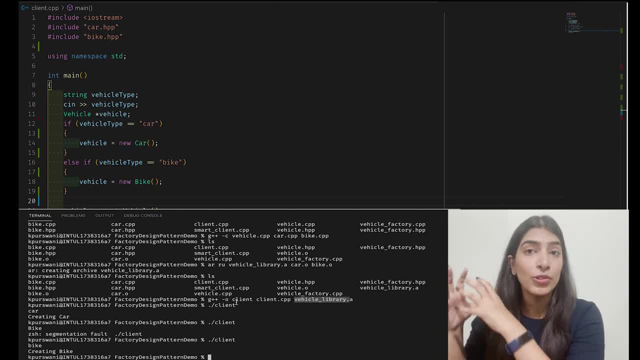 tightly coupled. our client should not be bothered with what we are doing with our library, right? so now what we are going to do is we are going to create a factory. what does factory do? in general, factory means creation, right, so it will take care of the entire creation. 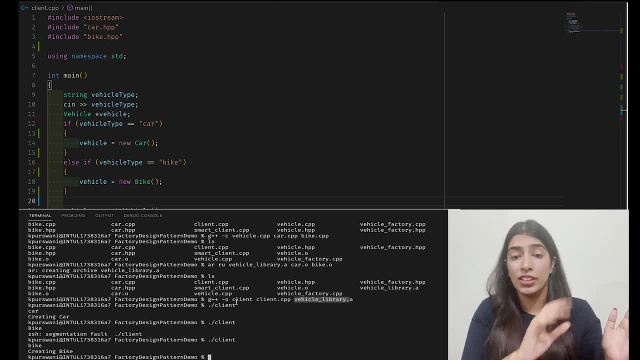 logic without exposing it to client. so client will not be bothered, it will just use vehicle. so that was the interface. that is the base class right. it is not bothered, it just takes the input, car, bike, anything, you just pass it, it is going to use it. so the creation logic is no more exposed to client. 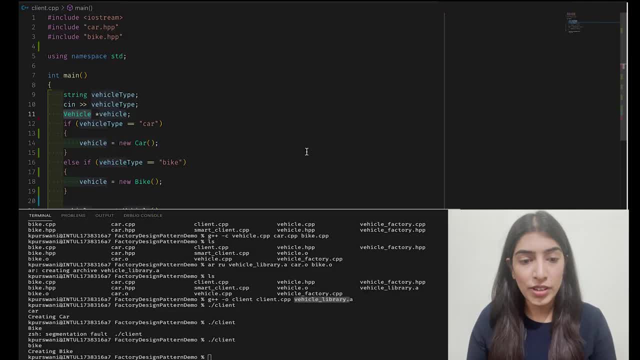 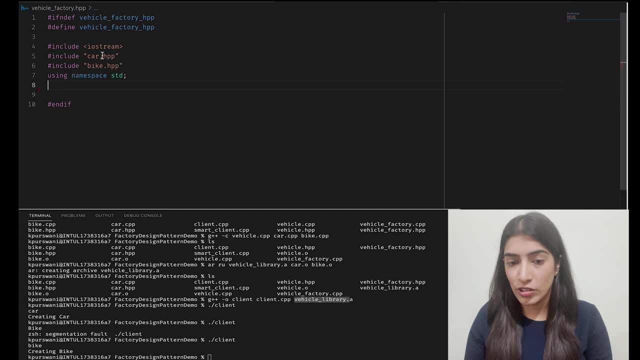 right. so now let's do this and see: okay, we are going to create a factory. now you can see, i have a file now: vehicle factory. right now it is including carhpp, bikehpp. and now tomorrow, if i want to make any changes, i just have to make changes in this factory. what i'll have to do, i'll. 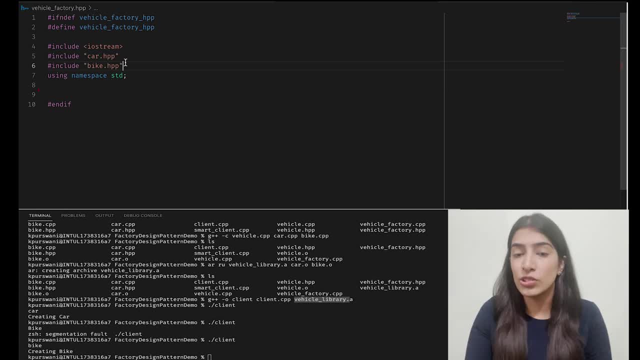 just have to include either the bus or tempo or anything to this particular file. okay, so i'm now going to write the class vehicle factory machine and i'm going to write one function over here that is going to return a vehicle and the function name is get vehicle. i'm going to give you input as a string, which will be the type, and i'll return the. 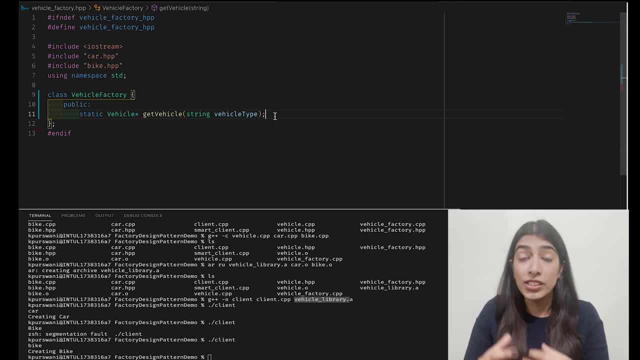 vehicle. i know you're wondering: why have i written the function as static? when we make a function the object of class. So if I did not make this function static, what would have happened is that I would have had to create an object of the vehicle factory class. I would have had to like: 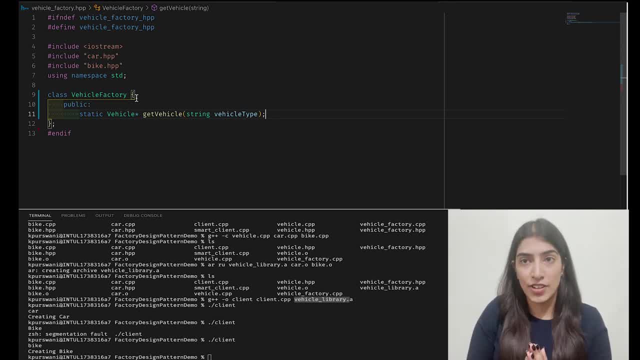 create an object- vehicle factory- and then access this particular function- right. But if the only purpose of this factory is to get the vehicle, it is just easier for me, like this, that I don't create any object. I can then access the function using the class itself. I don't need an object of the. 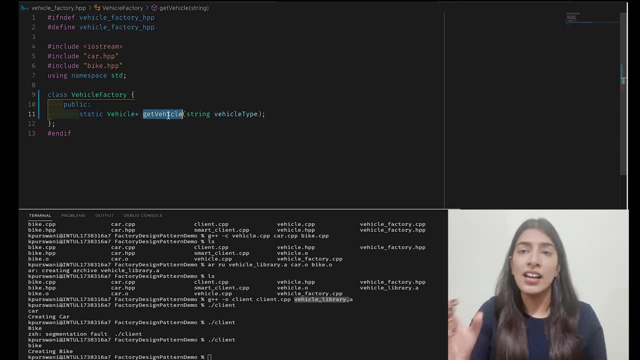 class. That is why I just made it as static. It is as simple as that. Otherwise, if you don't want to write it static, what you can do? you can do vehicle factory. you can create an object and then access the function. But this is the better way to do it because you don't need the object of 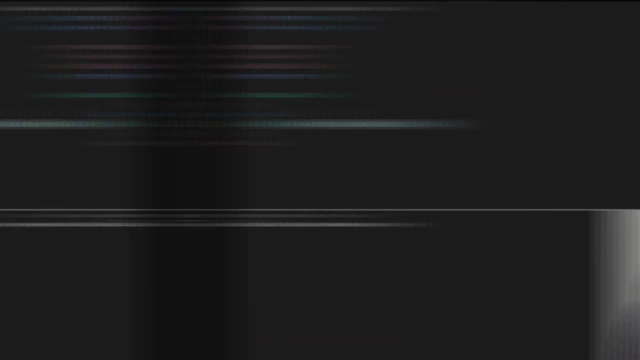 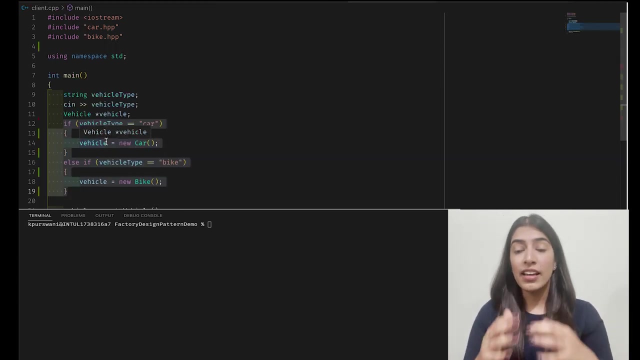 factory. you just need the function itself. It's easier this way, right. So earlier, whatever was there in client is now going to come into this function of factory. That means in client we had this if else condition, that car, bike and all is there. now it is going to move to factory and 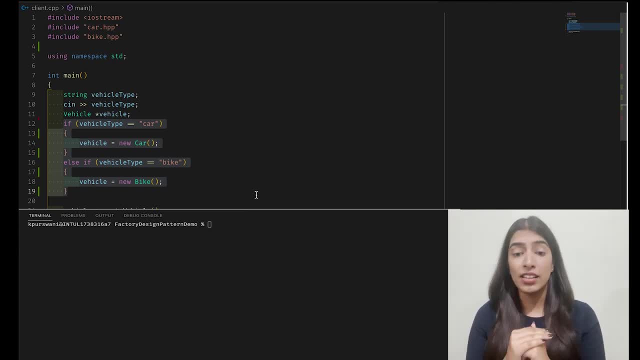 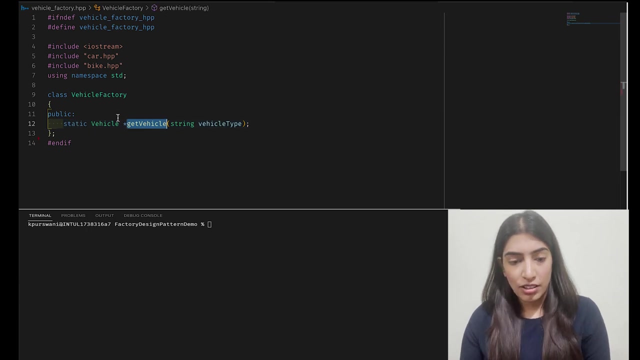 tomorrow, if there is bus Tempo anything, we need to add the if else in the factory itself, which is going to be part of library, and client will not have to recompile itself. So now let's write this function in the factory. So this is the function: get vehicle right. So let's implement this over here. 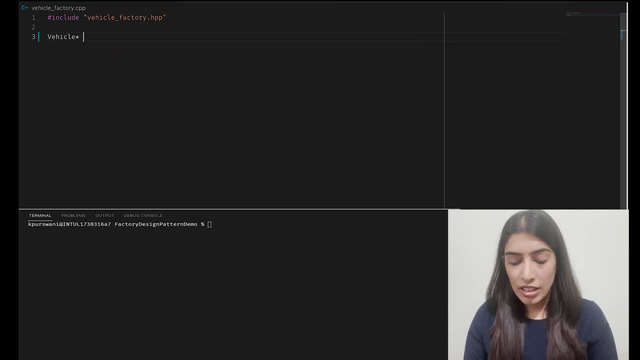 We are going to return vehicle pointer and it is part of vehicle factory, So let's just add that. Then I'm going to pass vehicle type to it, which will be a string, and now, whatever was there in the client, I'm going to copy paste the same thing. So I have created this vehicle. I'm going to take the code from: 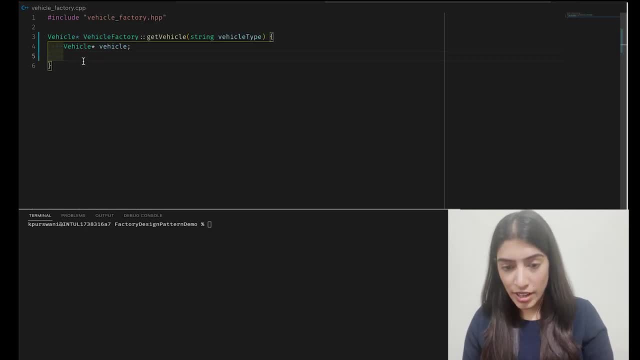 my client. I'm going to copy this code and I'm going to add it to my factory, Right, So? and I'm now going to return the vehicle. That's it. So this is what my factory does Tomorrow. I can just add the if else over here itself, I don't need to make any changes. 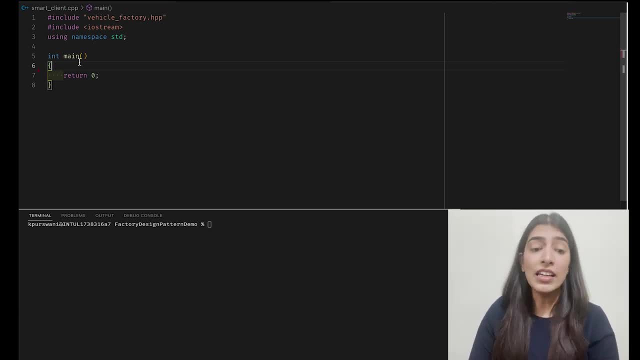 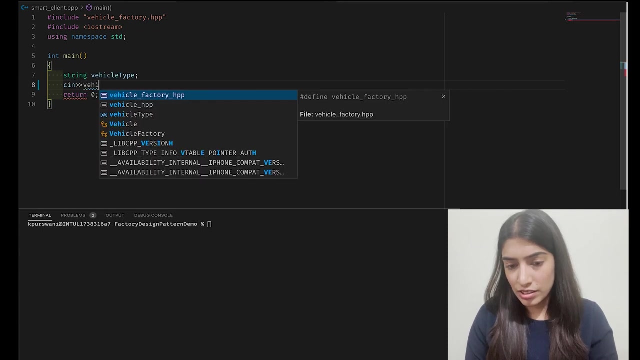 So now my smart client is the one that's going to use factory and it doesn't require the if else condition. So see how simple now the client will look. Okay, The smart client. all it needs is it needs. it still needs to take the input, which will be the vehicle type, Right, So we will take the 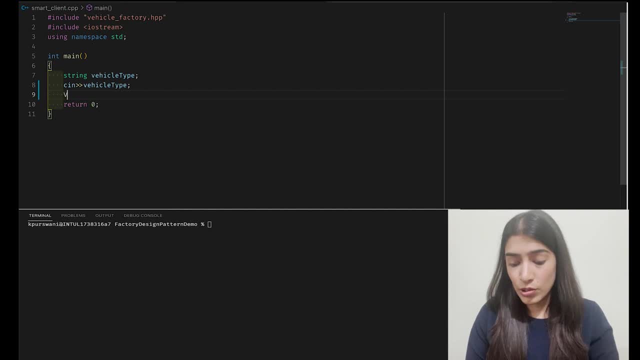 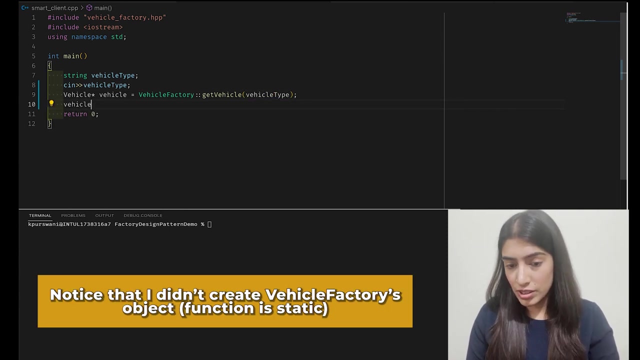 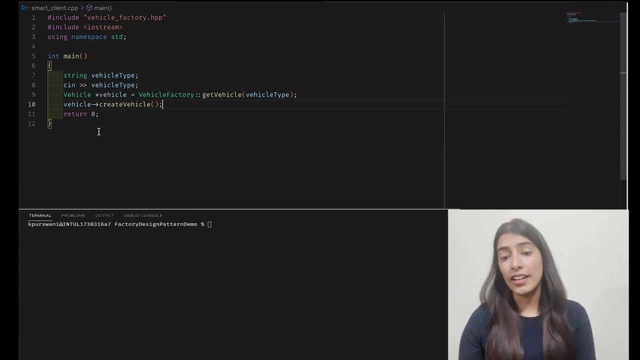 input And now we will use the factory To create a vehicle Vehicle factory. Okay, we just pass this vehicle type and now this vehicle. we just use it to create the vehicle. that's it. so tomorrow, if there are any changes in the factory, the client is not impacted. 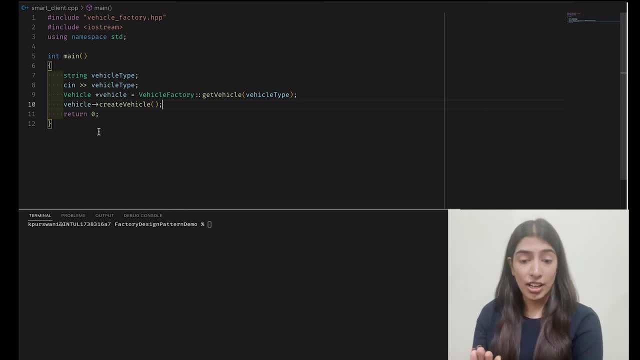 the client code does not change. it works like a chart. now for the demo purposes. let's actually do it. let's create the library including the factory and pass it to a smart client and see how easy it is for smart client to work now. ok, so now I am going to compile, just like 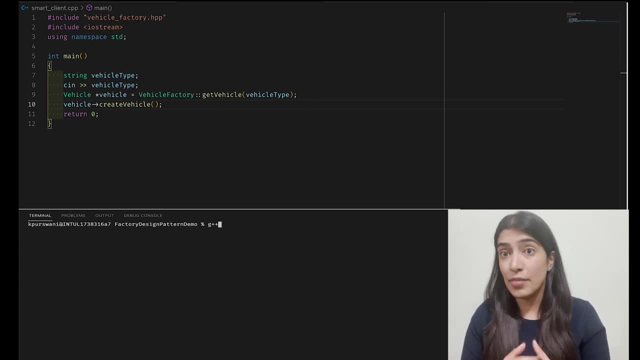 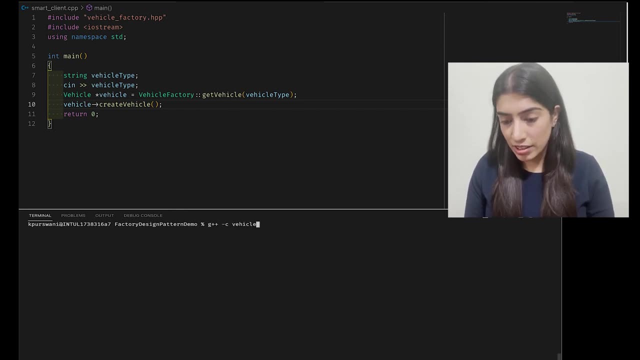 last time, but now, this time, I also need to add the library to my object files. right, so now I am going to compile, and this time I am going to compile my vehicle factory also. so vehicle factorycpp, carcpp, bikecpp and vehiclecpp- right, so now we can see the object. 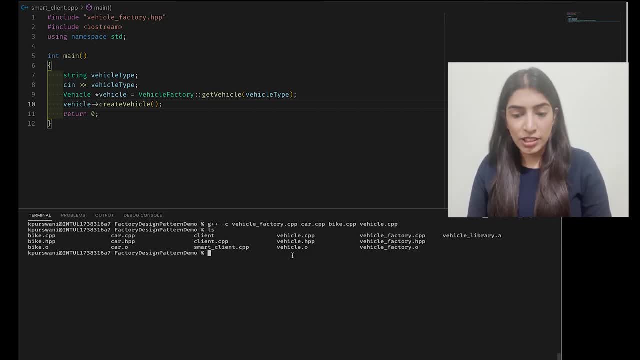 files must have been created here when vehiclecpp is created. so now we can see the object files right now. what we are going to do, we are going to create the library out of all of this. I am going to use the same library, I am going to call it vehicle librarya and I 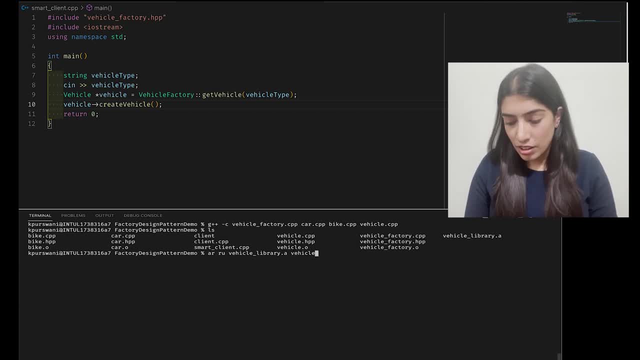 am going to put vehicle factory car object file. I am going to put cars object file, I am going to put bikes object file, right, so we have the library now. vehicle factory- vehicle librarya is there now. let's link the smart client with this library and we are going. 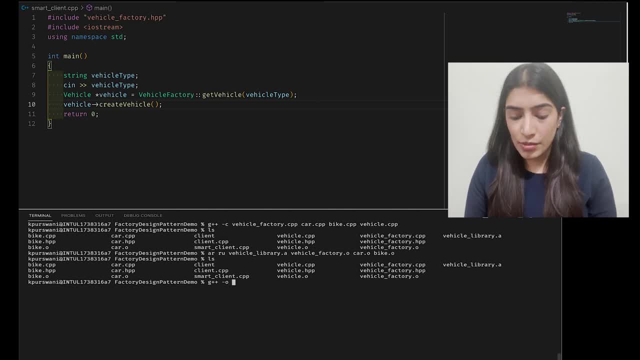 to create the library and let's see so g++-o, I am going to name the executable as smart client itself because it is very smart, and I am going to use the vehicle librarya. let's run this smart client and see if I give the input as car. it is creating car if I give. 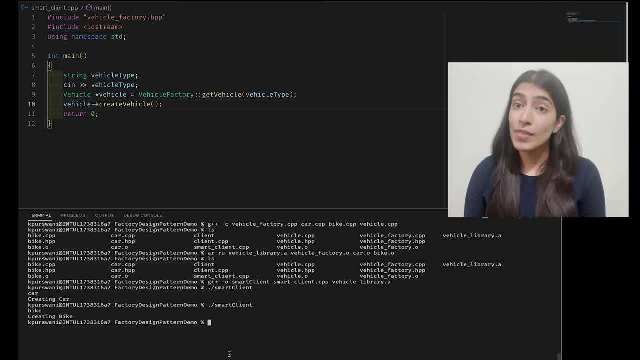 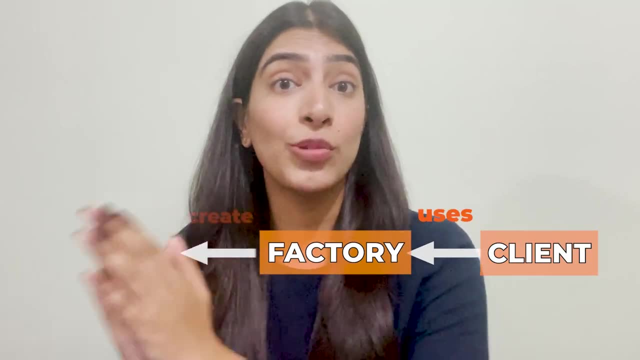 the input as bike. it is creating bike. so this client is so smart. just for a recap, what would we do when we use the factory class after this, our client uses the factory to create the product. so now things are very decalcified right now. we are going to create the factory. 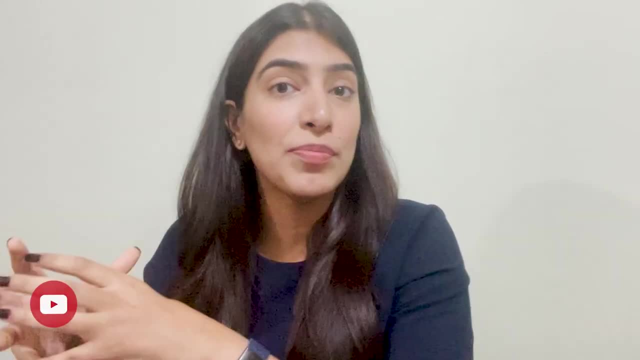 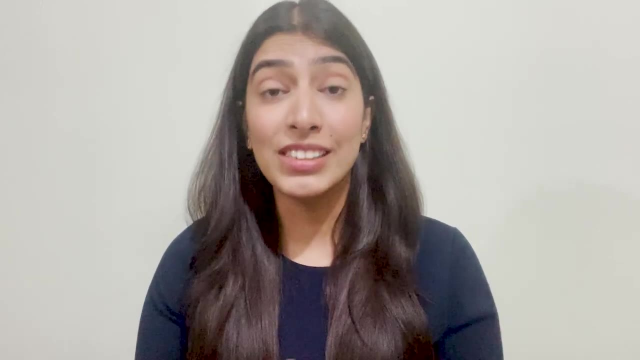 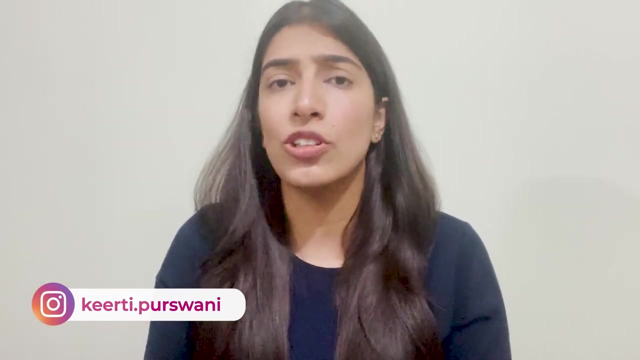 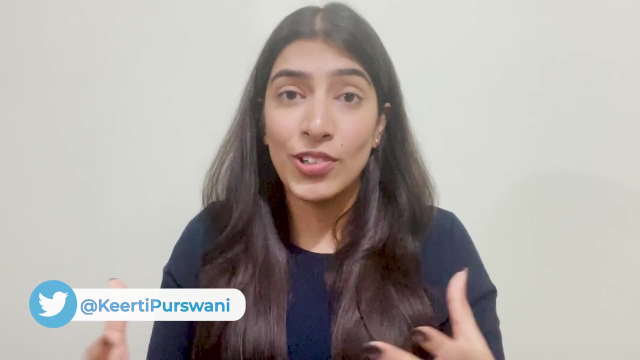 class and we are going to create the factory class. and we are going to create the factory class without any ICAppled. our client doesn't need to know how the implementation is happening, how the object is being created. it just tells factory that I need to create this, to create it and give.